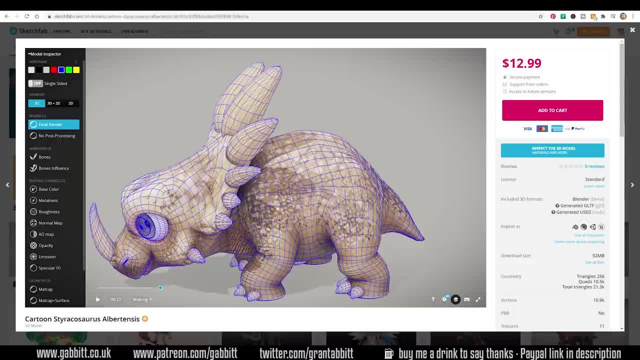 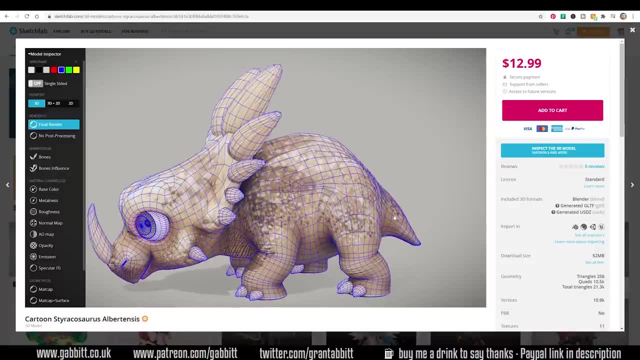 information on that, But you can see how the topology flows in different directions when it hits one of these poles and they're crucial to understanding topology. So we can easily analyze and look at these models to influence our own understanding of topology. Let's quickly take a. 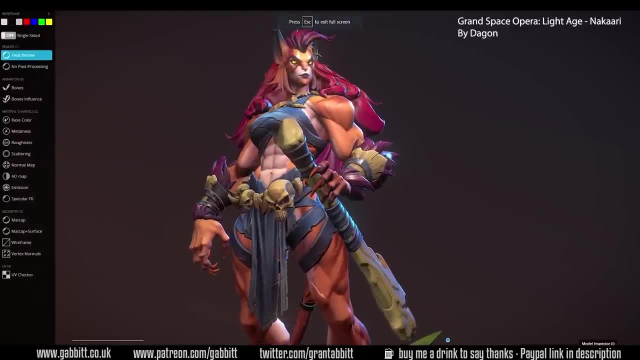 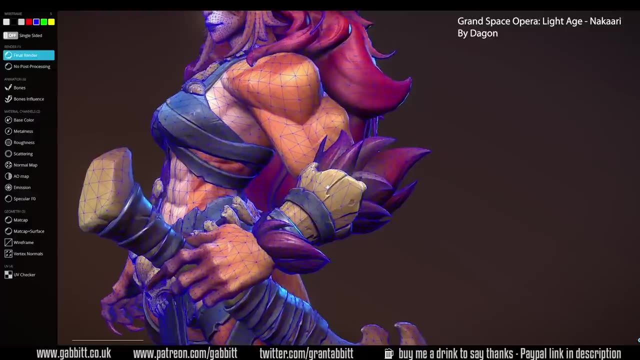 great looking model. Let's maximize that and analyze it as well. Quickly put on the wireframe and see what's going on. Now this might look like it's not a quad based mesh, but that's only because it's been triangulated for using game engines and things like that, because everything gets converted. 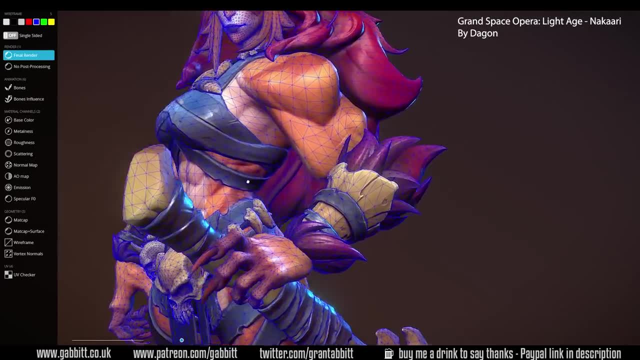 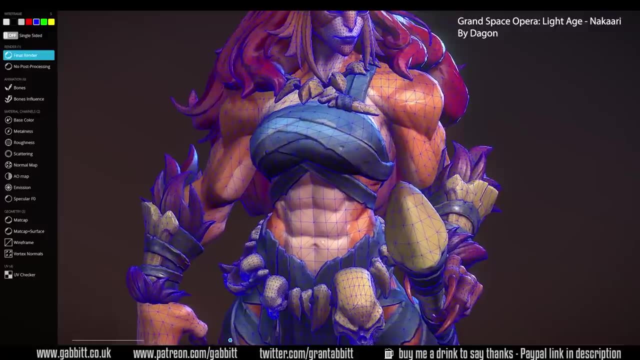 to triangles in the end. So don't get confused when you see a mesh like this and assume they're a bad model or something strange like that. Like I say, it's just been triangulated so you can actually see the quad based mesh going through here, but each of the quads is then split into a triangle. 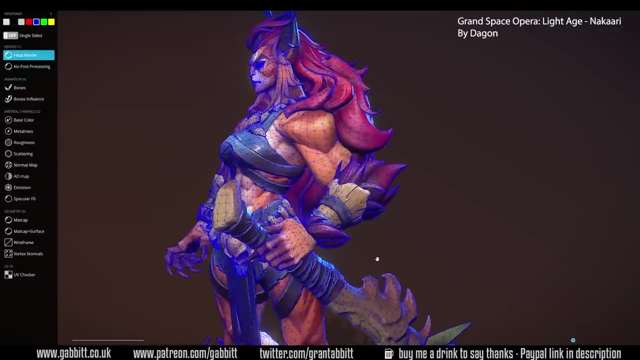 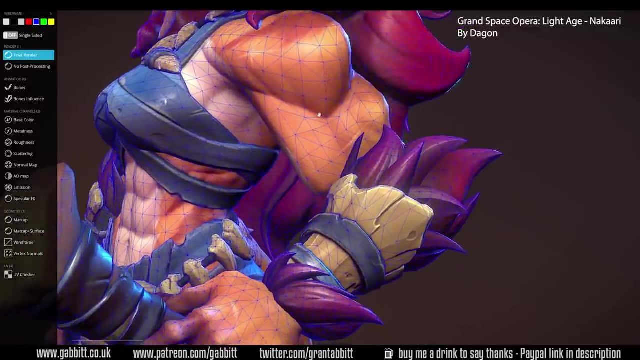 and you can see how the topology flows in different directions. You can see some of the detail there and this is great for learning how other artists treat and deal with topology issues, For example, the edge flow around the shoulders here and how the quads move and adapt to the shape, And you can 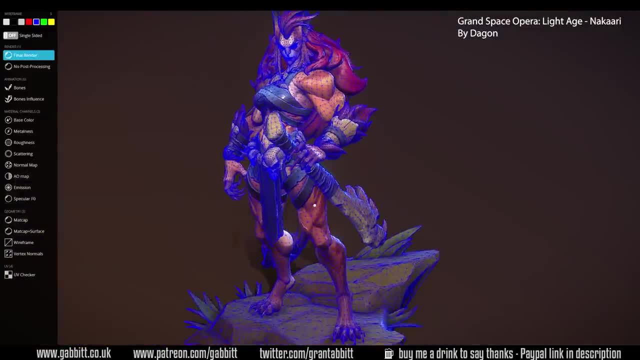 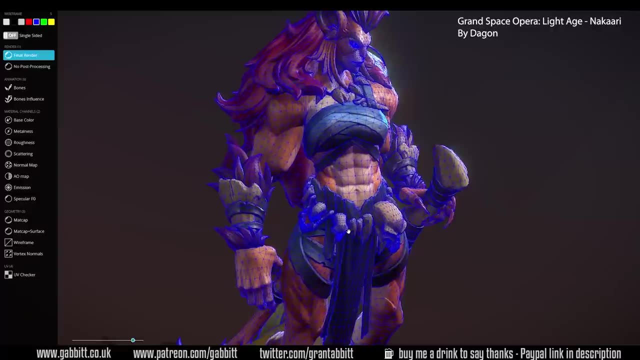 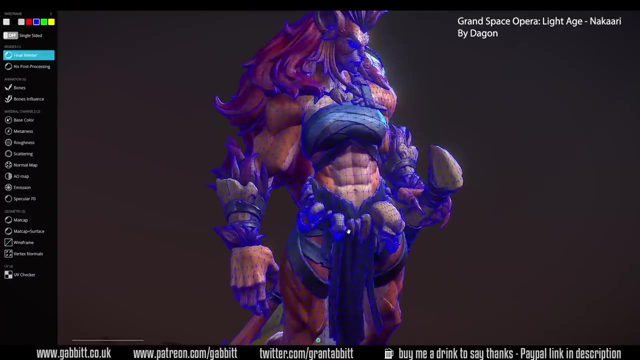 see there's a pole there which changes our topology flow. This is also very useful for thinking about how high or low poly you need to go with your models. I would say for a game model this is a very low poly model, but it's still very low poly, so it fits within that threshold that you have. 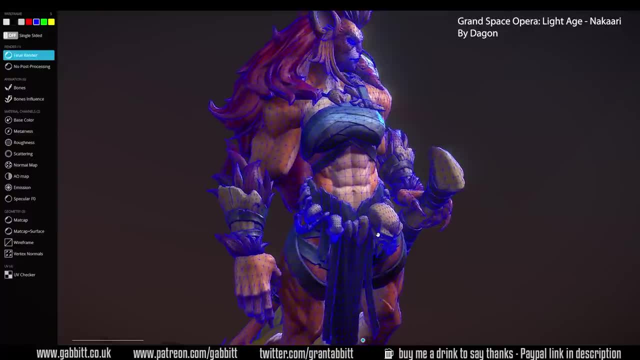 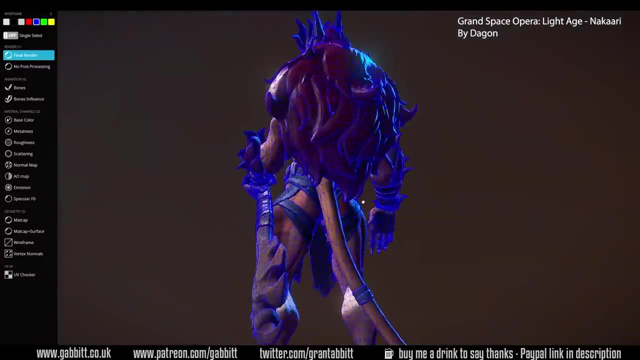 for games, which generally is getting quite high these days. But, you'll notice as well, there's no wasted topology, no extra faces that we don't need, so it's really useful to be able to look at models like this and analyze them in this way. Incidentally, you can also see things like the: 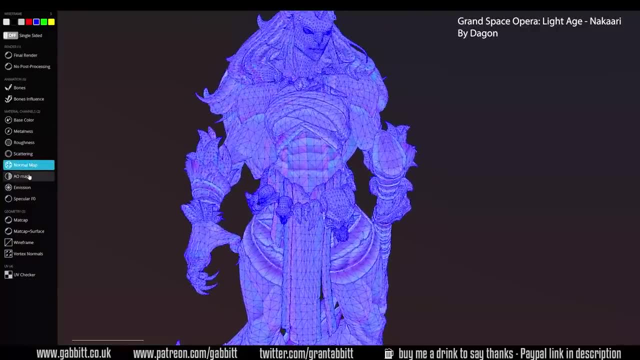 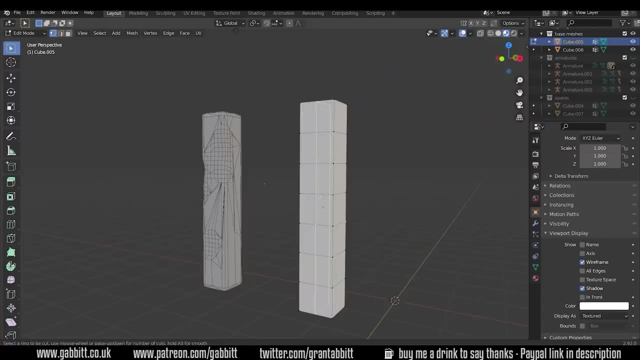 metalness maps and roughness maps to learn more about those. So hopefully you've looked at my re-topology- a detailed guide video- and you understand good. topology tends to be in quads. Quads are much easier to model with. cut through. add extra loops. 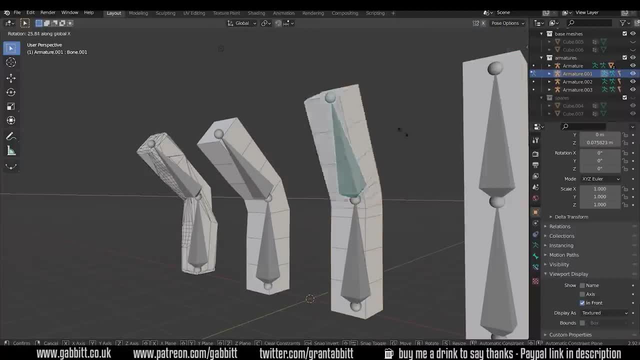 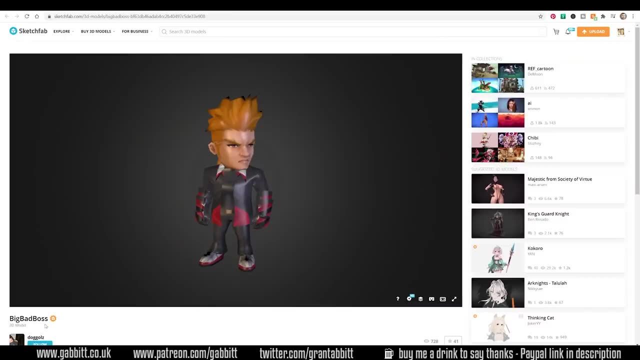 they work well with subdivision surfaces and so on. But we don't always have to model in quads and it does depend on the model and what it's going to be used for. Take this model, for example: Big Bad Boss. It's a lovely low poly model, looks really great. Let's have a look at the model. 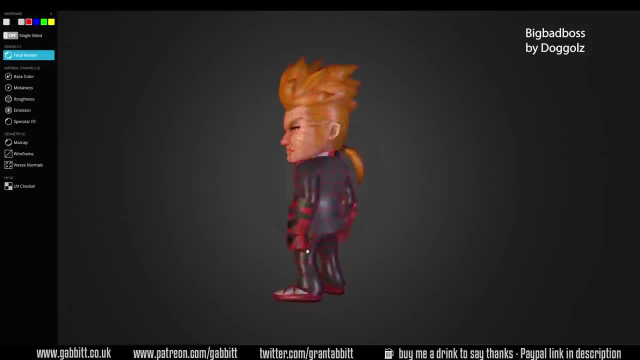 inspector and see what's going on with the topology. So we can see it's really low poly, this one suitable for a mobile game, but it's not actually all in quads. If you look at the topology you can see that the model is in quads. if we look at things like the back of the legs here, 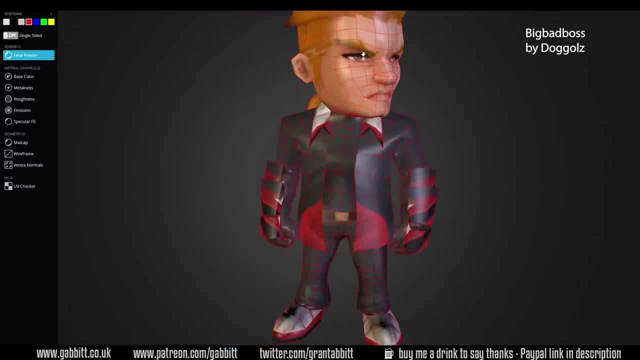 and the arm actually kind of intersects the body here, which seems strange, but it works really well. You've even got triangles around the eyes. So with low poly modeling like this, the most important things are to keep the silhouette from all angles. So that's the outline that you can see here. You 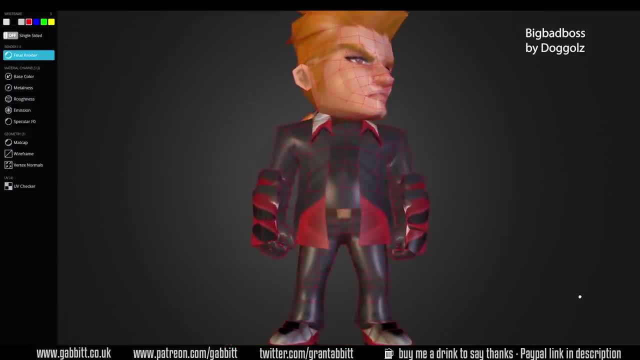 can see when I go round, it keeps its shape all the time, so that silhouette, the outline, as we call it. So it's just the right amount of topology. Take this jacket, for example, if I look from the base to it, but at no point do we lose that silhouette. So if there wasn't this cut down here, you might. 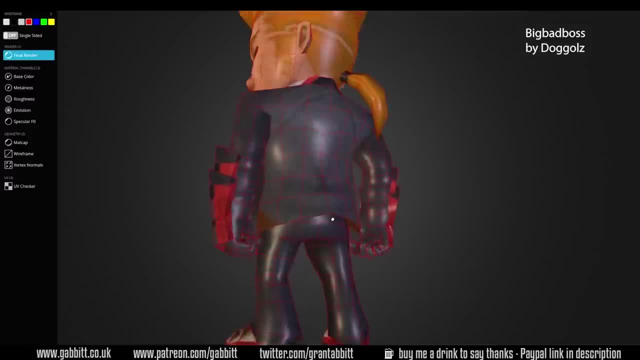 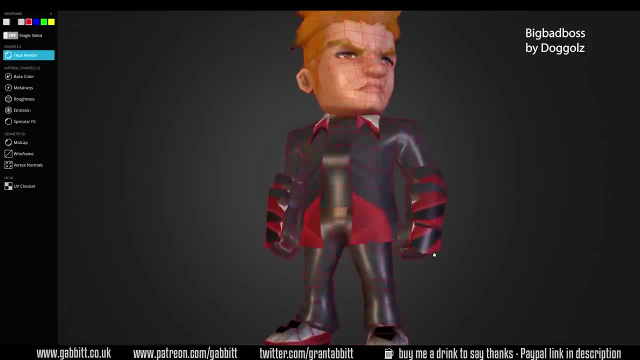 have an even lower poly version and a big face across here. We'd see more of a kink in that jacket and more of a flat shape going across here. So this is just the right amount of polygons and it's really kind of optimal. Notice as well, we haven't got the inside of the jacket, it just cuts. 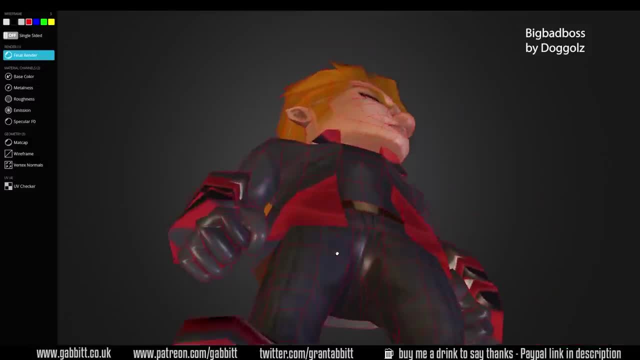 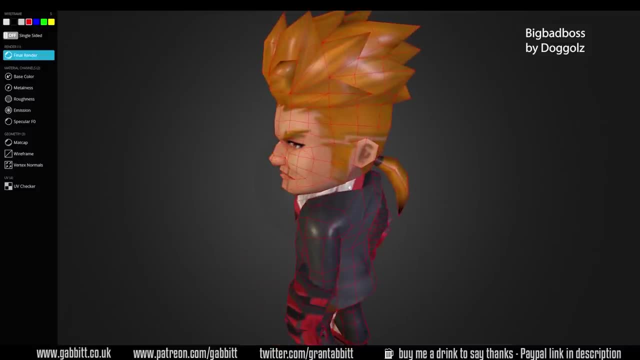 off in here and joins to the trousers at the bottom. here The collar is also interesting how it sort of overlaps just on this bit but then joins up to the rest of the jacket up here. So keeping the integrity of the silhouette whilst also keeping the polygons down. Not only that, 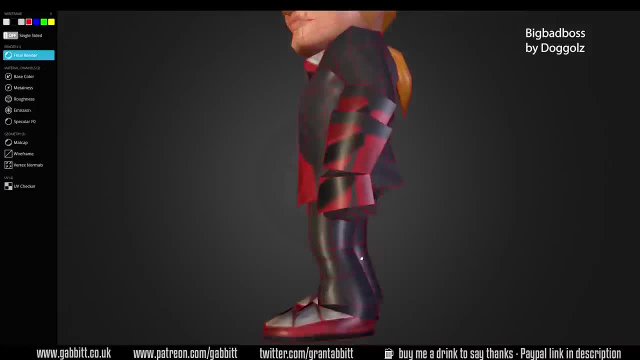 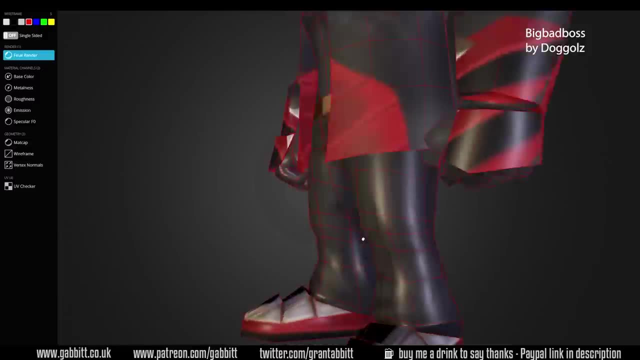 we need to also think about animation. So, like I referred to earlier, in the knees here we've got these triangles at the back and an extra cut at the front here to help the animation, And that should deform really nicely and animate well. So topology isn't only about making the 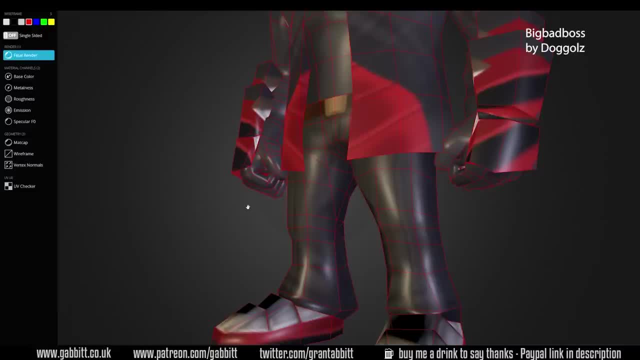 shape look good. it's also about how it animates, So it's a good idea to look for examples of low poly characters that are animated as well. And again, you can see my retopology, a detailed guide, for more information on animation with topology. Now, another great resource that I've used before. 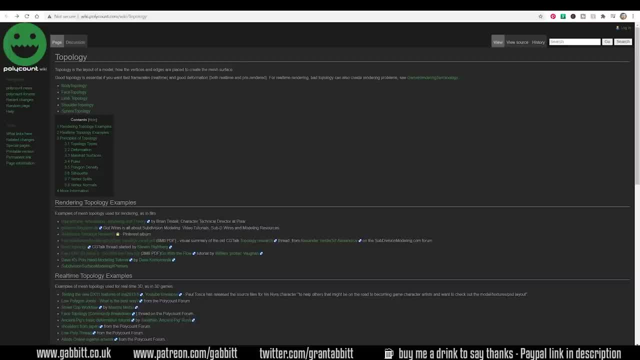 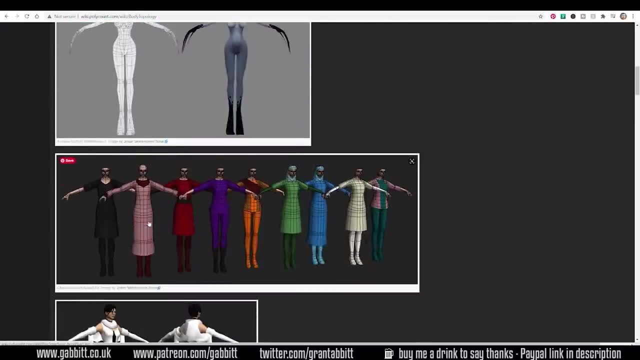 is the polycount wiki. I'll put a link in the description. Now, this is quite old, but it's still really, really useful. It's got examples of topology. so let's go to body topology, for example, and you can see. it's got lots of guides, pictures for you. 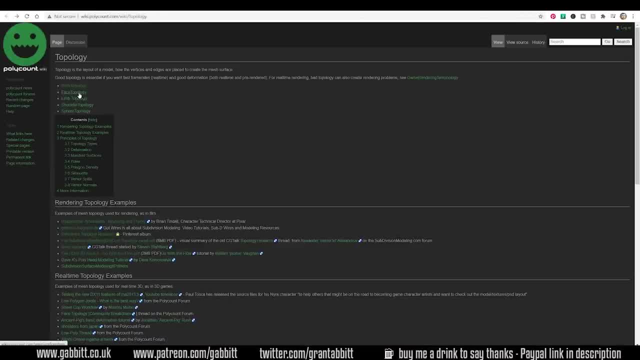 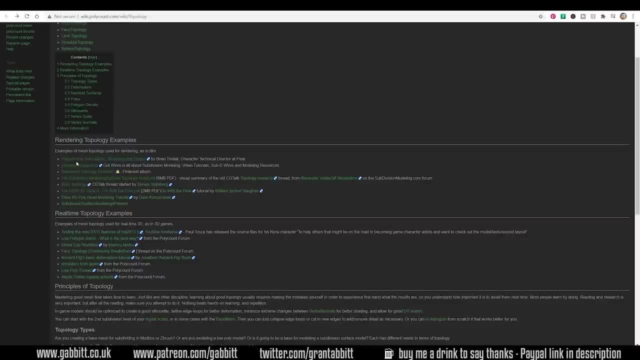 with really detailed, in-depth information, mainly focusing on the body, But if we scroll down a bit as well, we've got some great topology examples here. Some of these links don't work anymore because it's quite old, but take a look through each of them, because the ones that are still there. 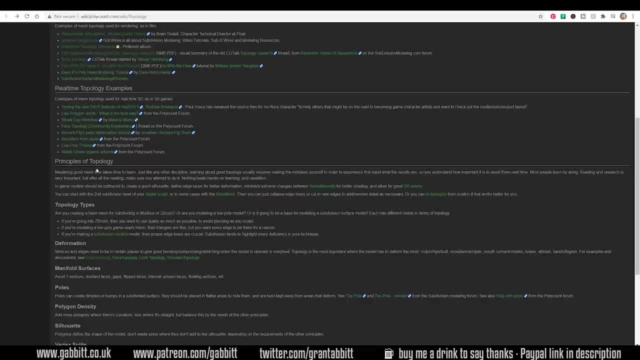 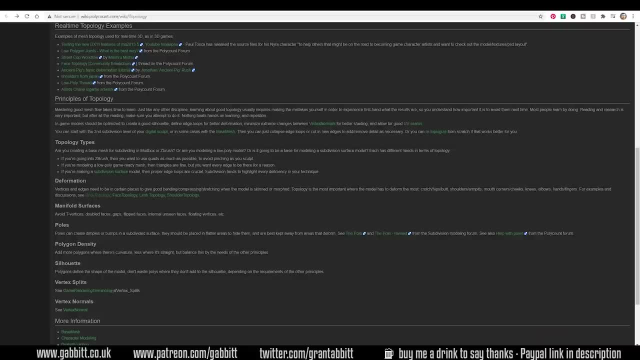 are really useful. Also, it's got this section on principles of topology and it's got some really useful information there. nice and simple, but it defines each of these things that are worth looking up, And there's poles, which I've been talking about earlier. There's even a low poly thread. 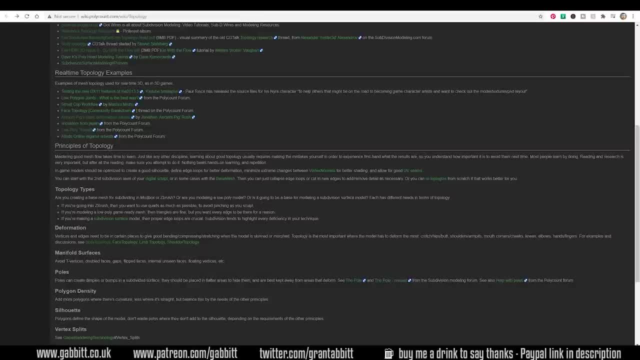 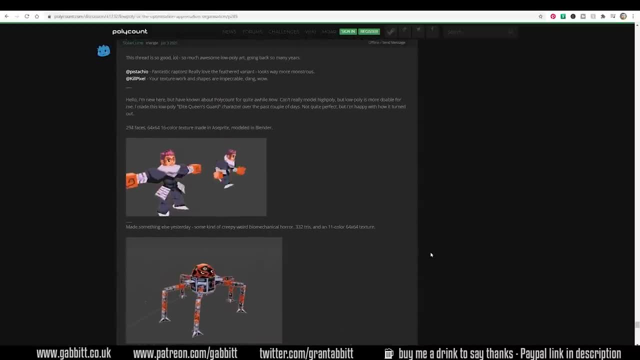 on the poly count, There's the poly count forum, which is a great forum well worth taking a look at, which is still relatively active today, and you can post your models and maybe get a bit of feedback and ask questions about topology. So that's my guide for getting better at topology. So a few. 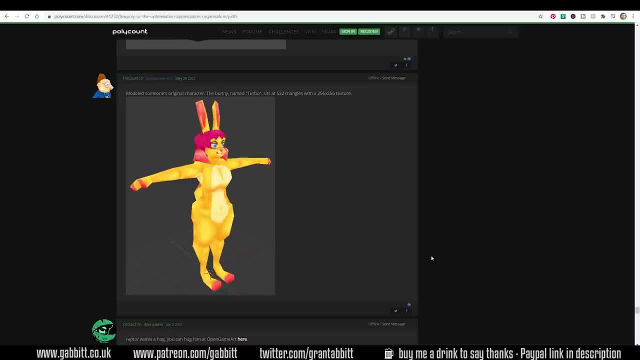 resources on my channel. We've got sketchfab to really analyze and look at other people's models and we've got the polycount wiki and forum for looking at really detailed, in-depth guides and examples which we can learn from there. So thanks for watching and I hope this helps. 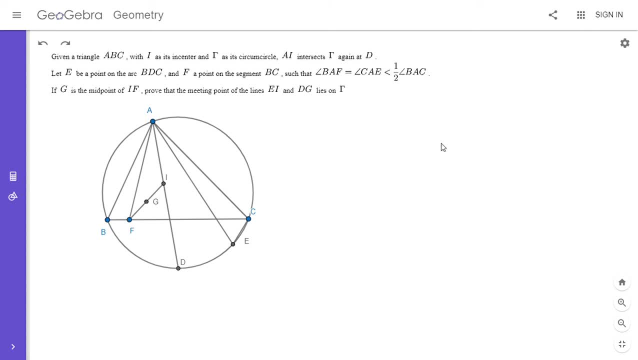 Hi everyone. it's Michael, So I have a very illustrative problem for you all today. This one was on the 2010 IMO exam, So it wasn't just a candidate problem, it was actually on the test And it was the second problem on the exam, so it was of medium difficulty. So if you'd like, 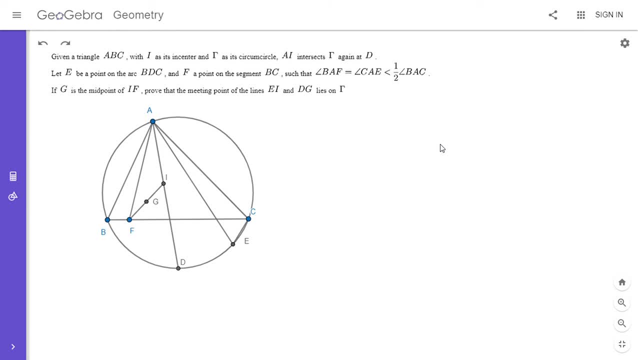 to try to solve it. feel free to pause the video. All right, so I'm going to go over my solution. So we have a triangle: ABC, I is the in-center and gamma is the circumcircle. AI intersects gamma again at point D. Let E be some point on the arc BDC and let F be on segment BC, so that angle BAF.